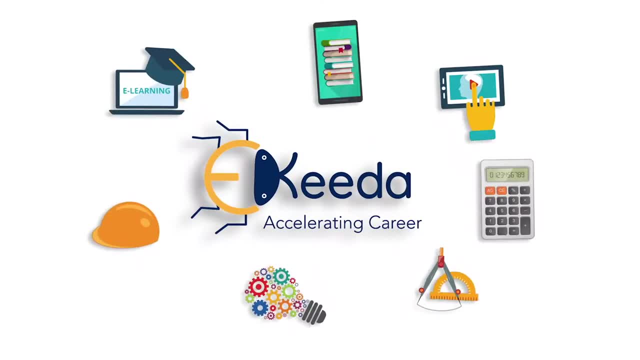 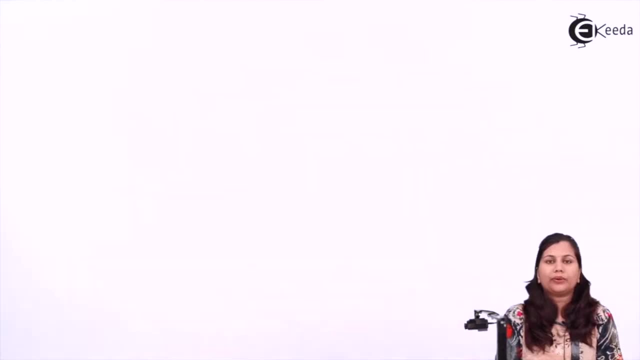 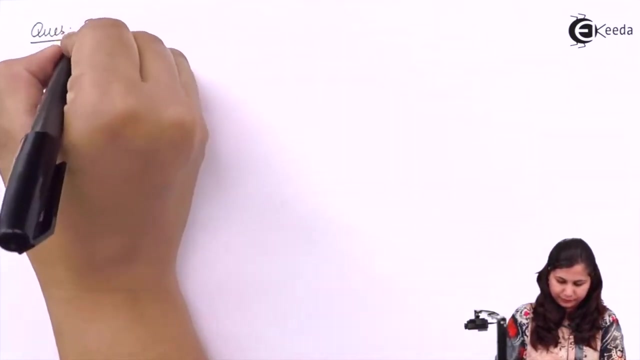 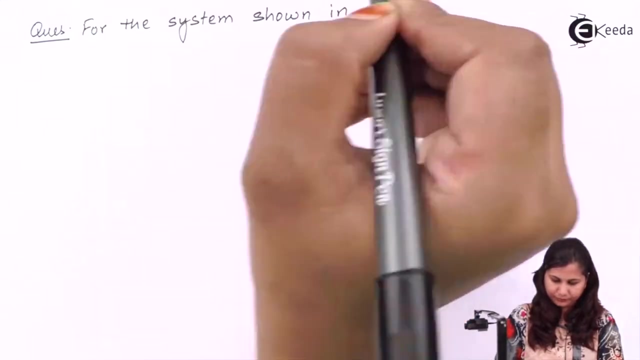 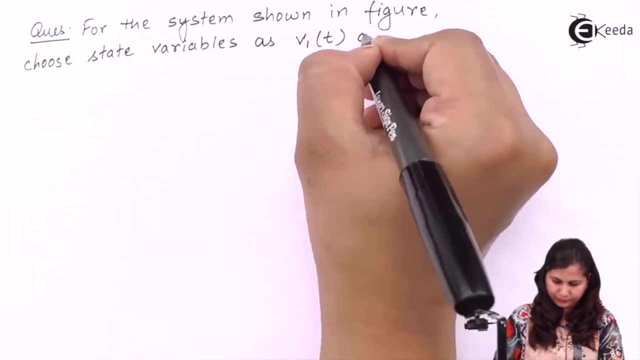 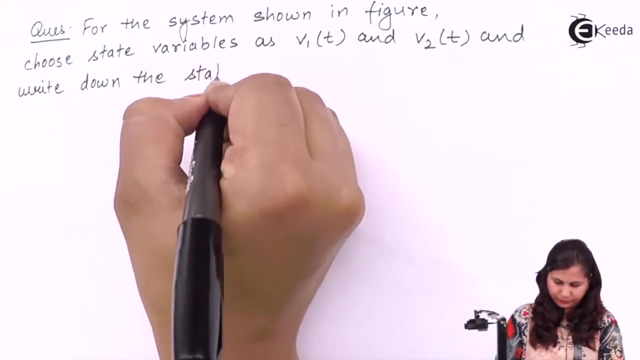 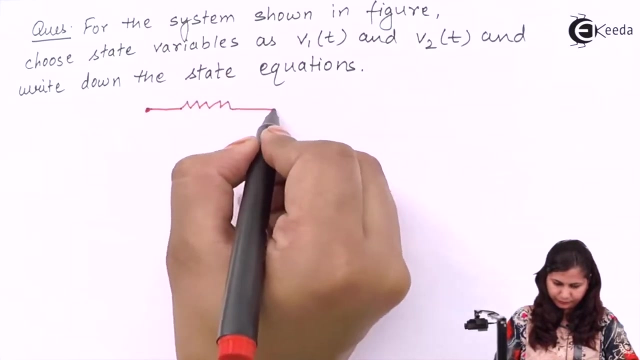 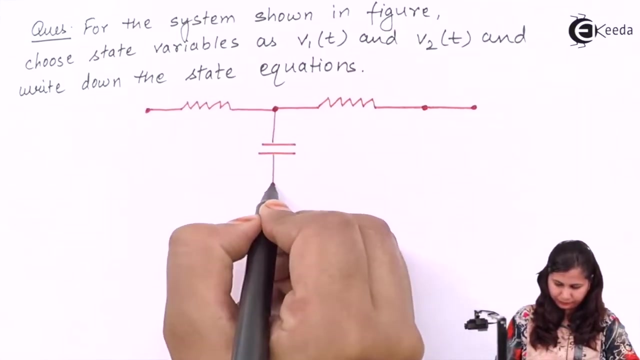 Hello friends, in this video we are going to solve a problem on how we can find out the state-space representation of a system. So let's take a problem. We are going to solve a problem on how we can find out the state-space representation of a system. 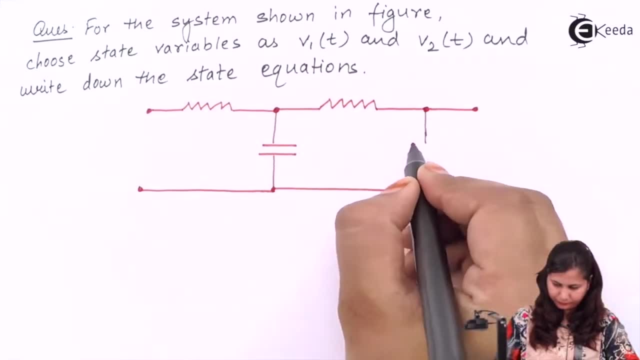 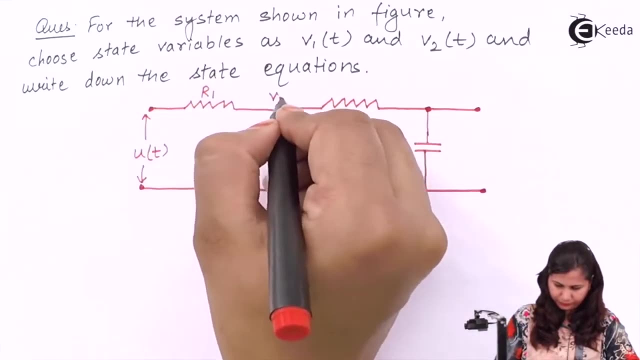 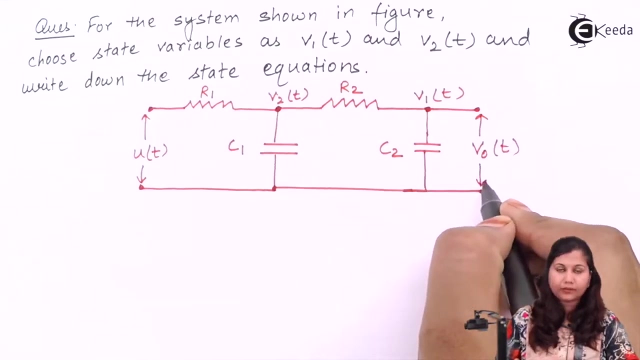 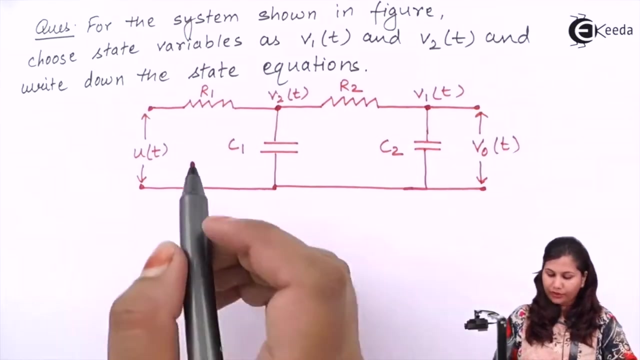 So our problem is to find the state-space representation or the state equations of this system, And we have to choose the state variables as v1, v2, v3, v4, v5, v6, v7, v8, v9, v10, v11, v12, v13, v14,, v15,, v16, v17,, v18,, v19, v20.. 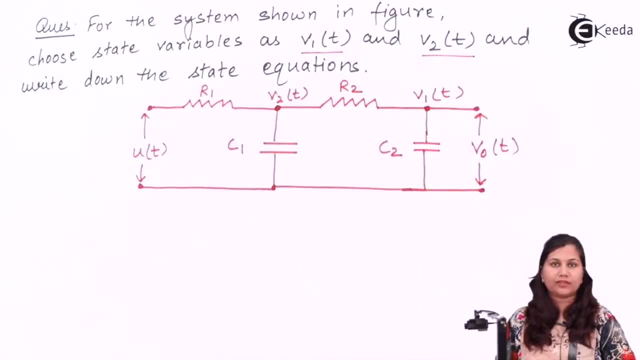 So our problem is to find the state-space representation or the state equations of this system. So these are the two state variables and using these two state variables, we have to find out the state equations and the state model of the system. So let's solve this problem. 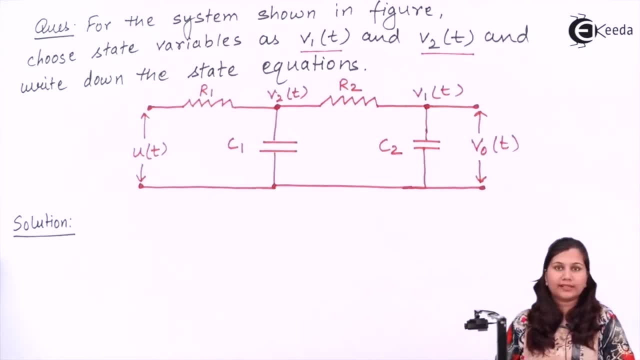 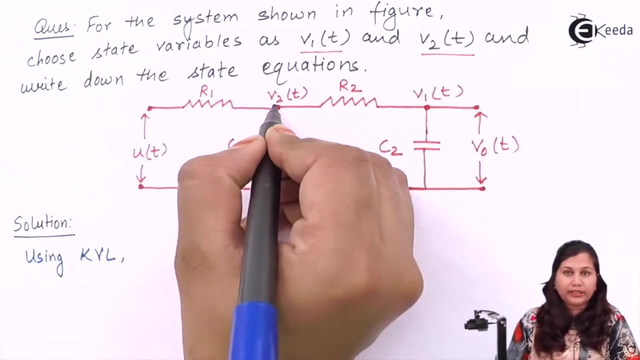 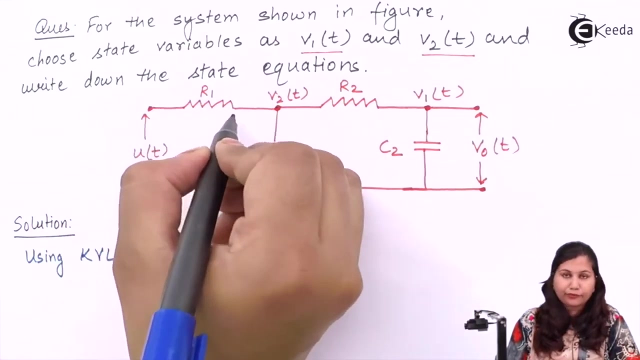 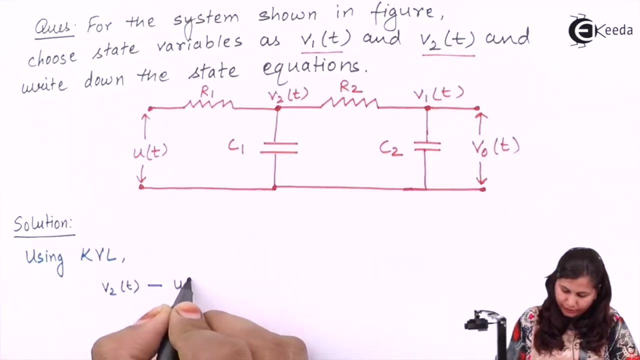 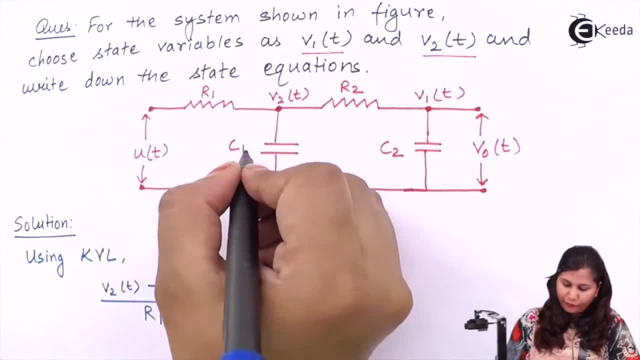 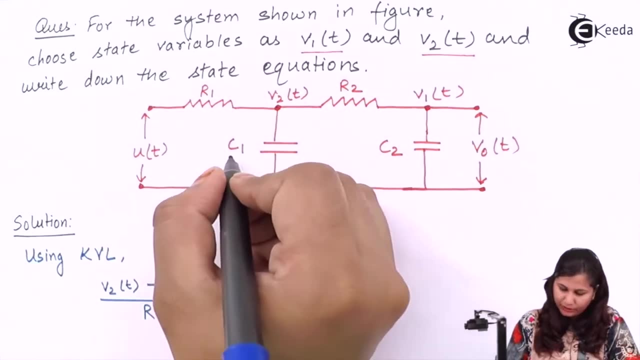 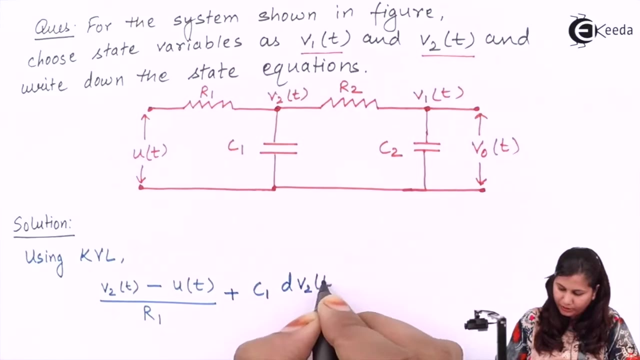 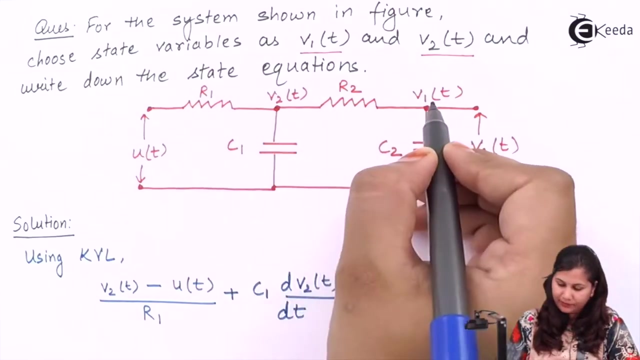 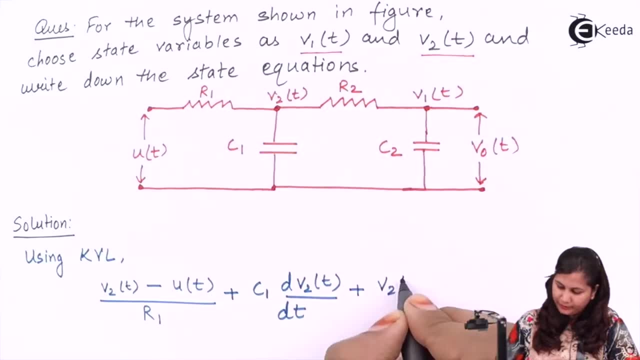 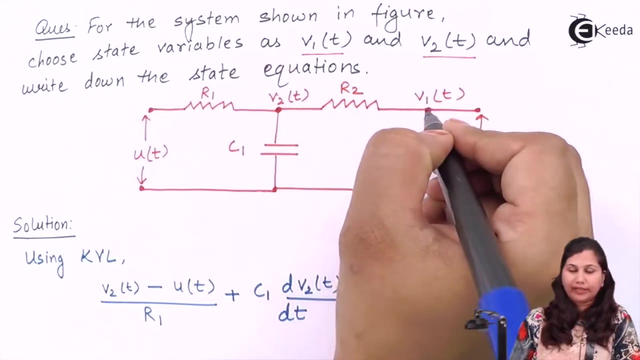 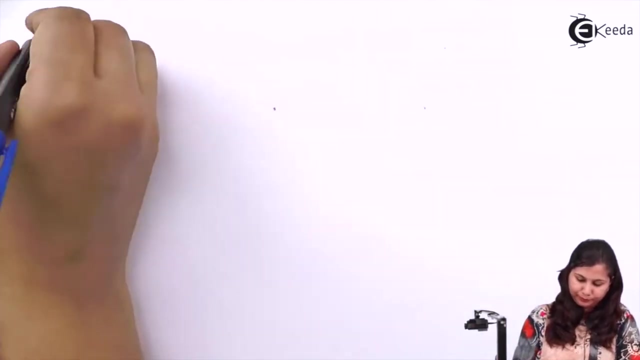 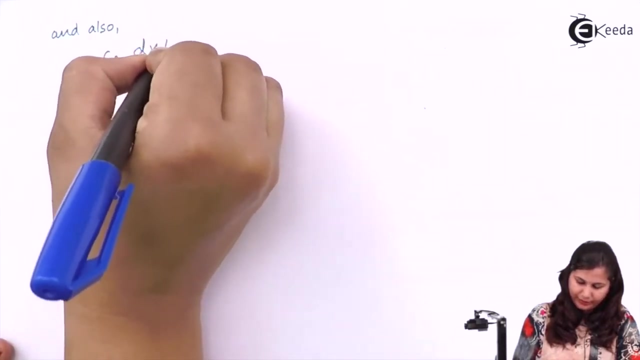 So we will have v2t minus v1t upon r2 equals to 0.. So this is our first equation. Now, also at this node, we will write the KVL, We will apply the KVL here and write the equations. So our equation will be: and also we will have C2 d, v1t by dt, the current across the capacitor C2. 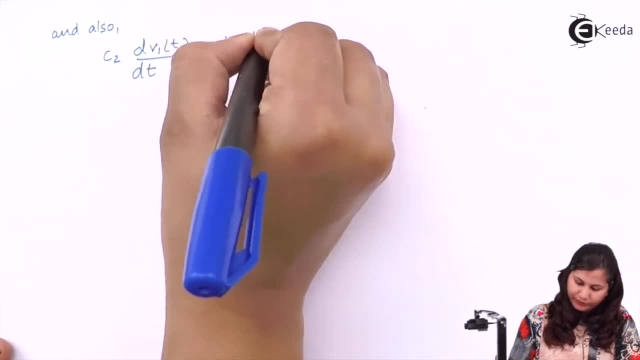 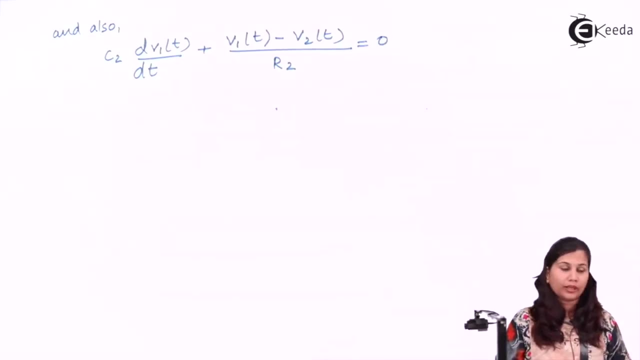 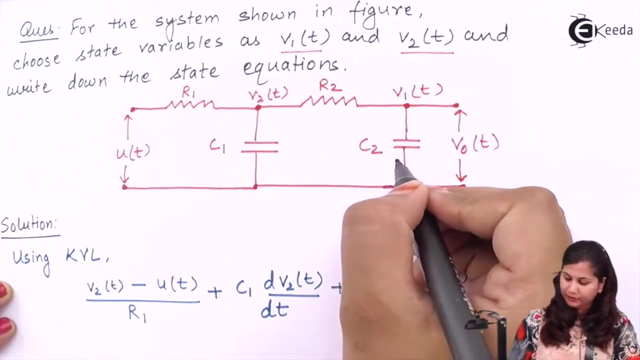 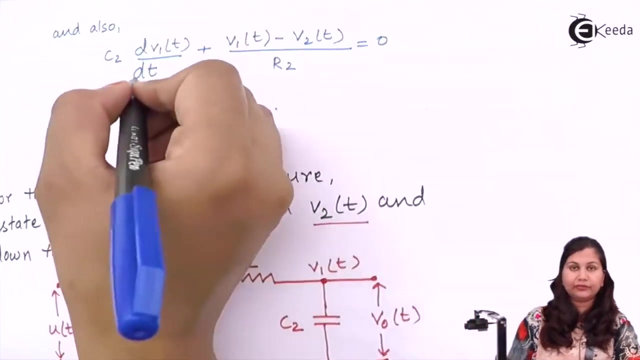 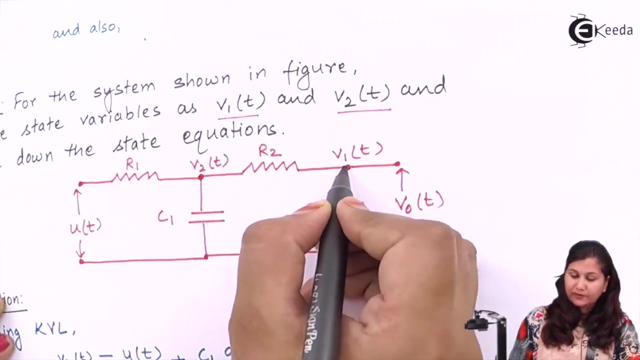 plus v1t, minus v2t upon r2 equals to 0.. How we have written this, For at this node the voltage across this capacitor will be or the current will be d C2 multiplied with d v1t by dt. We have written here, plus the current across this resistance will be v1t. because we are writing the. 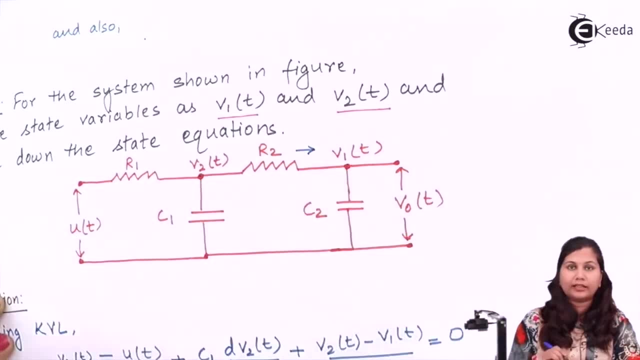 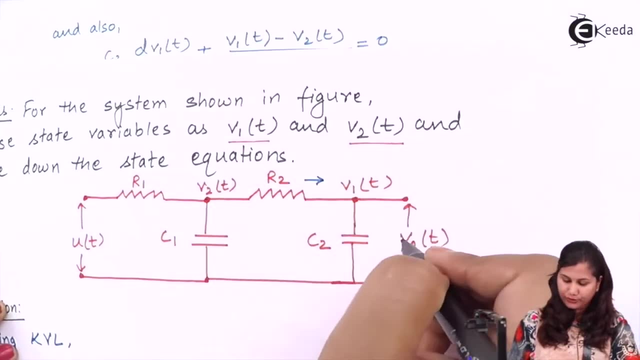 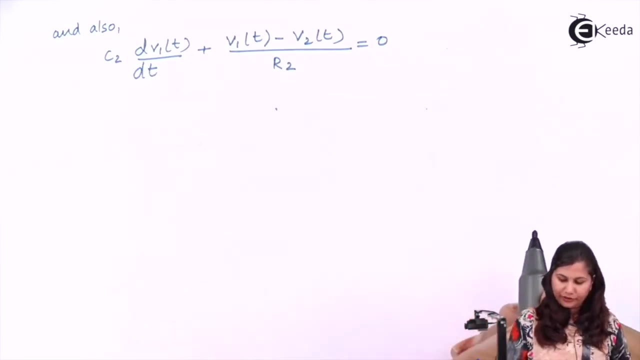 node equation for this node. So we will consider the current in this direction. So it will be v1t minus v2t upon r2 equals to 0. And also we have this v0t, it will be equals to v1t. Now rearranging, we have two equations. First is: 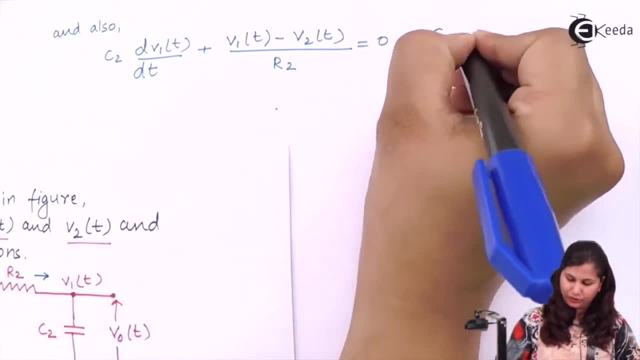 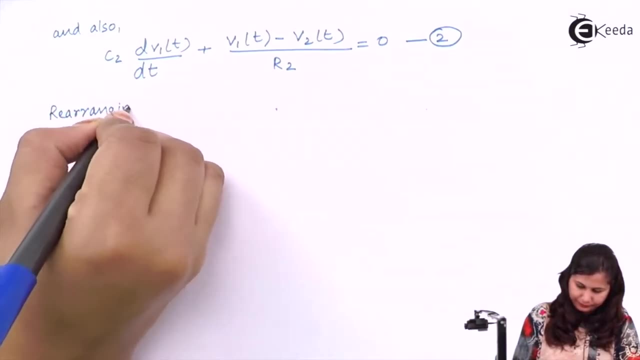 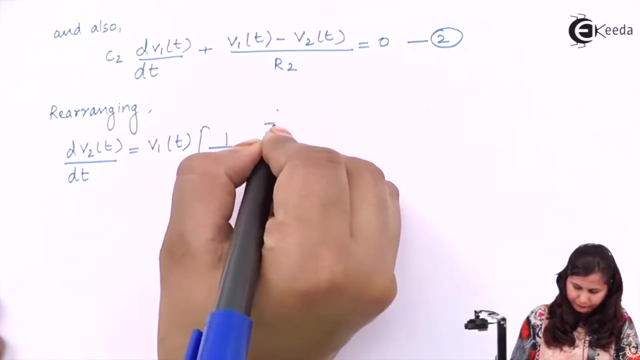 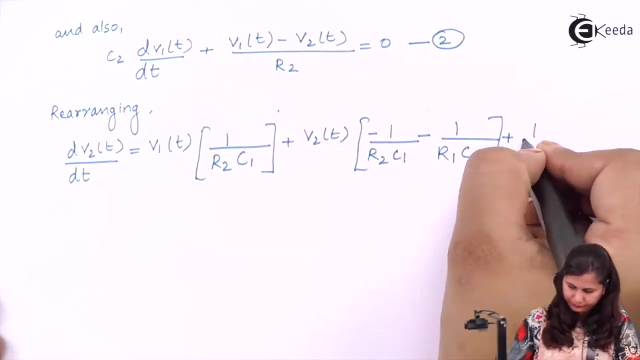 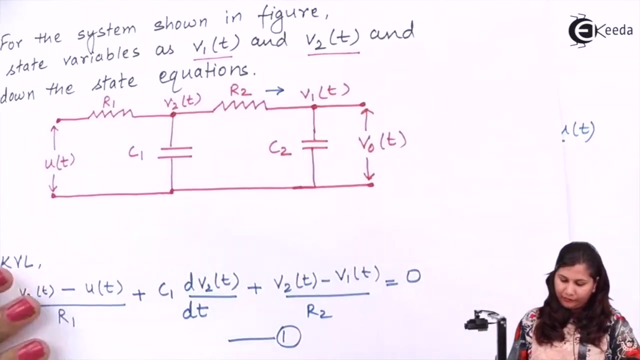 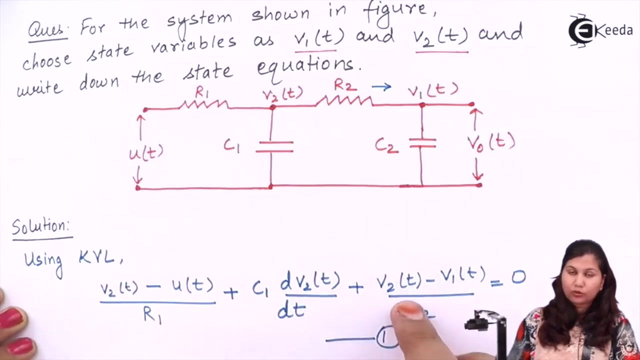 this equation and second, is this equation So rearranging? we will get this equation. So what we have done We have. we want to get the value of this d? v2 by dt. So from here, d? v2 by dt will be: this will goes to the right hand side and this term will also goes to: 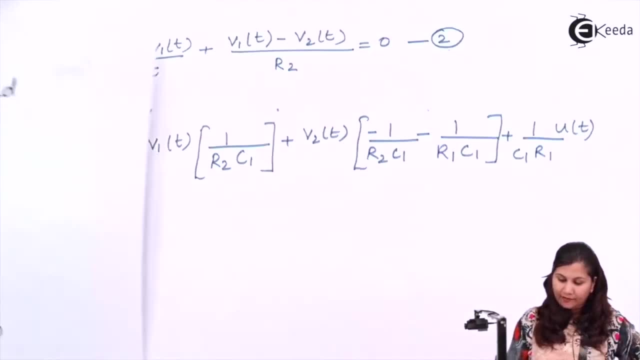 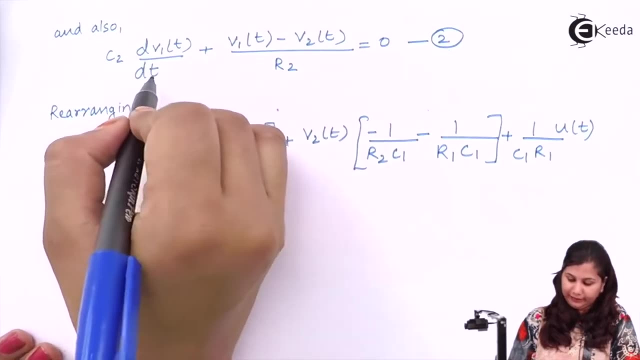 the right hand side, divided by C1.. Then we have put this value here. from here we have taken the value of v1, this d, v1 by dt. So we have taken the value of d, v1 by dt. So from here we have. 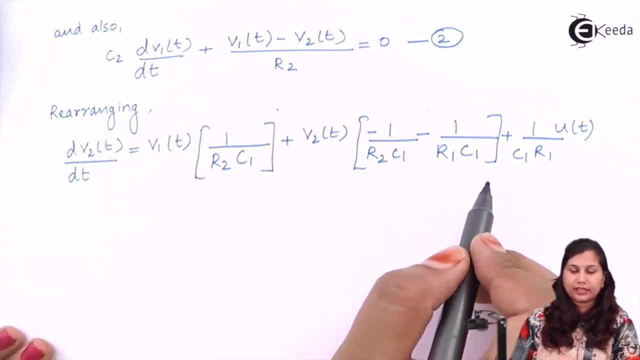 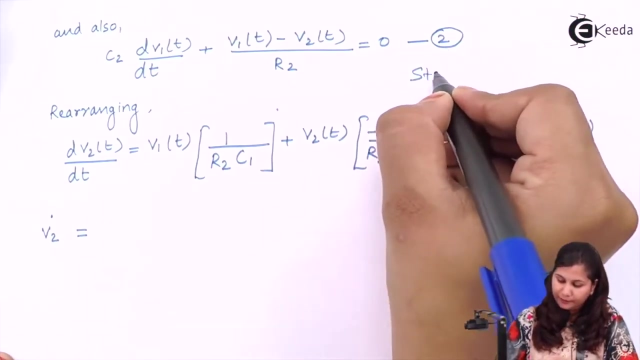 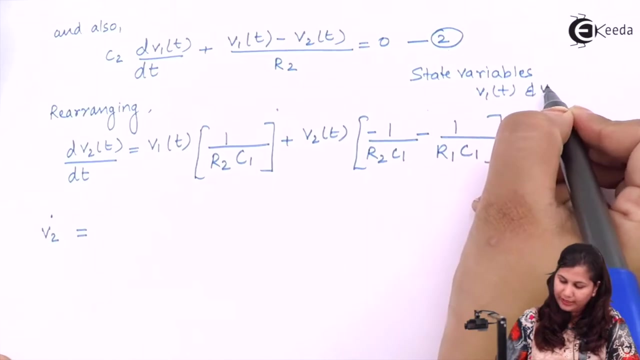 done this equation, This, so we have our fed evacuation of v1 and v2 by dt and we have substituted here in this equation. So we have got the value of dv2 by dt, or we can write it as v2- dot in terms of the tool state variables, because we have to choose v1t and v2t as our to state. 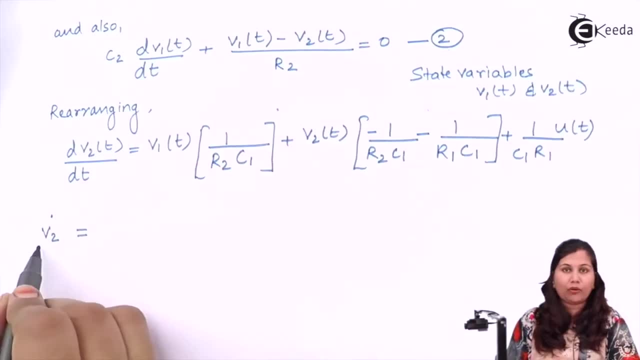 variables. So this expression is the derivative of the state variable. The state variable we are also using is v1c, equal to v1Bait. here And now to between these two values. we have followed some soma to come up here that we have first translated 2x. So if you took or if there were, 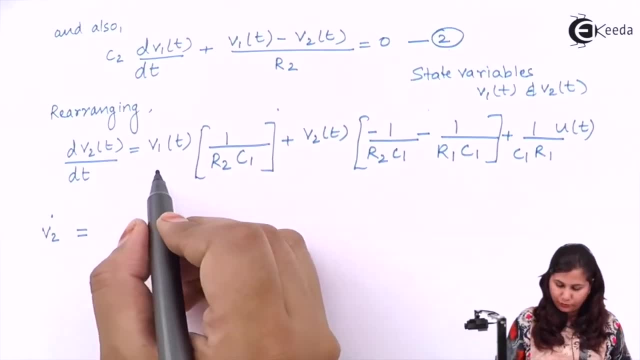 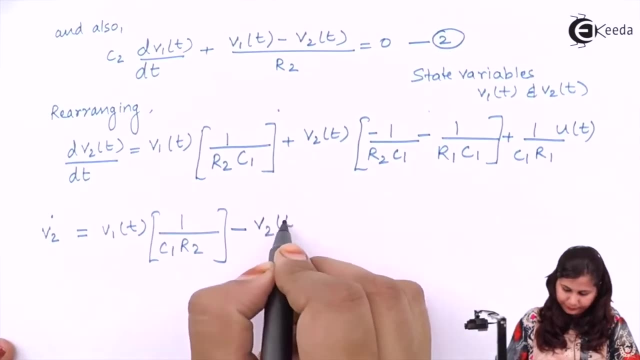 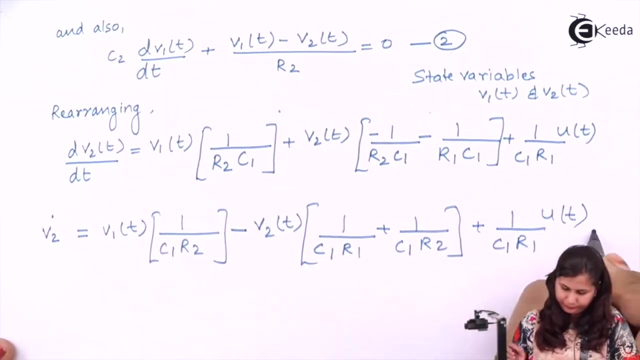 2x from the first equation, the state variable y of v1t and y how軽 a integrate. So that would state variable v2.. So this will be equals to v1, t, 1 upon c1 r2.. Okay, So this is the. 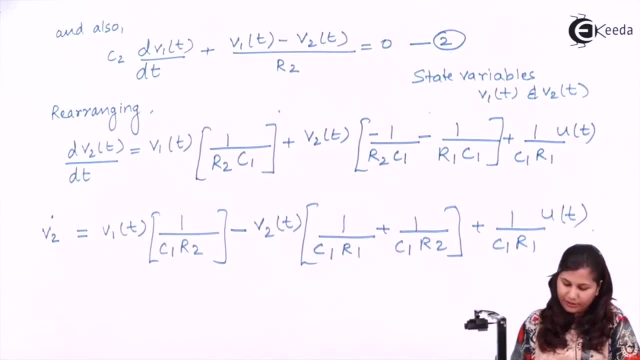 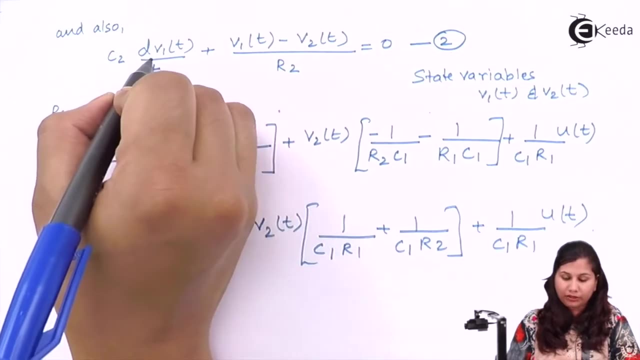 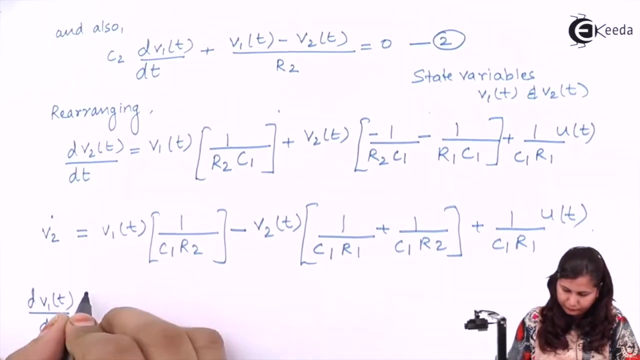 equation for v2, dot or the derivative of the state variable. Now here from this second equation we can get the derivative of the state variable, v1. So its value will be: this will goes to the right hand side, So it will become minus v1 t upon r2 c2.. This 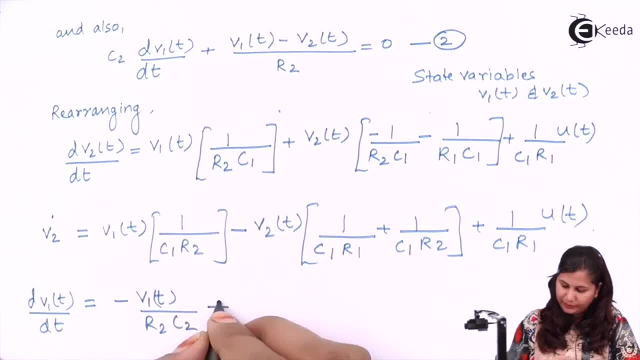 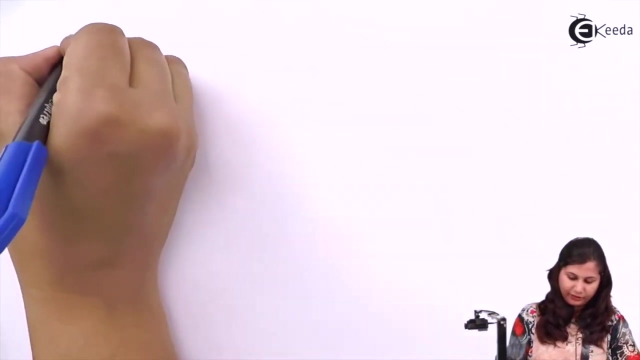 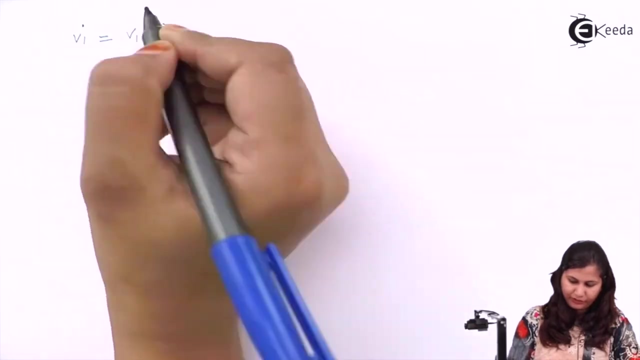 c2 will goes in the denominator, Then this will become plus v2 t upon c2 r2.. Okay, Mark this equation as third equation and when we solve this equation we will get our v1 dot. That is the derivative of the state variable v1, and it will be equals to v1 t, 1 upon From. 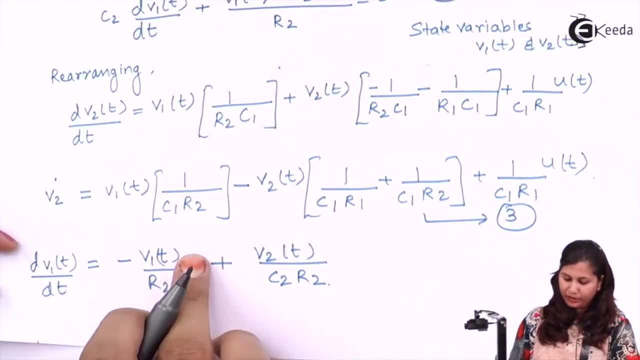 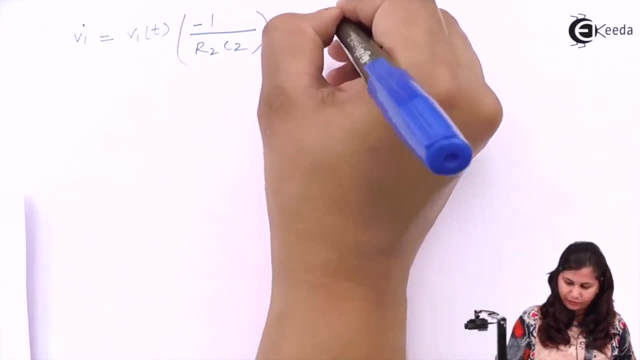 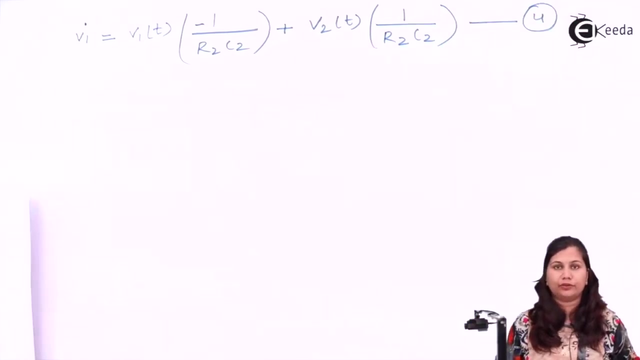 here it will be v1 t multiplied with minus 1 upon r2 c2 plus v2 t. So we have v1 dot multiplied with 1 upon r2 c. Mark this equation as fourth equation. So you can see that this third and the fourth equation, they are the derivatives of the. 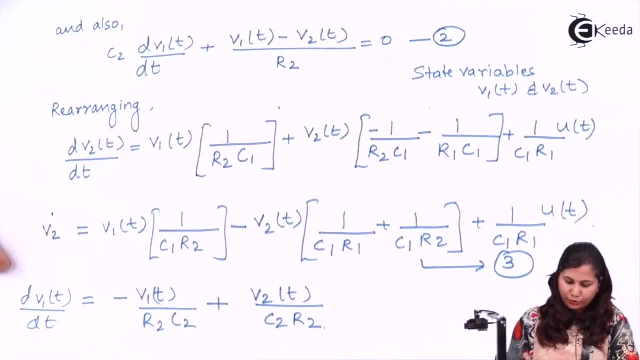 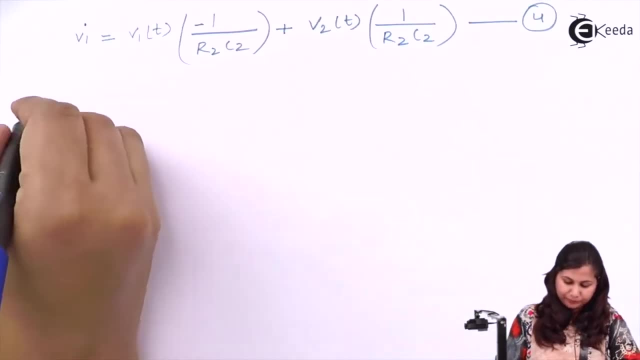 two state variables: v1 and v2.. So using these two equations we can find out the state equation of the system, So how it can be written. We have v1 dot, v2 dot, v1 dot. So we have: 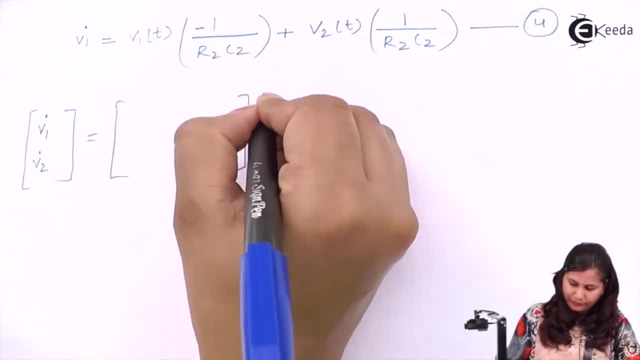 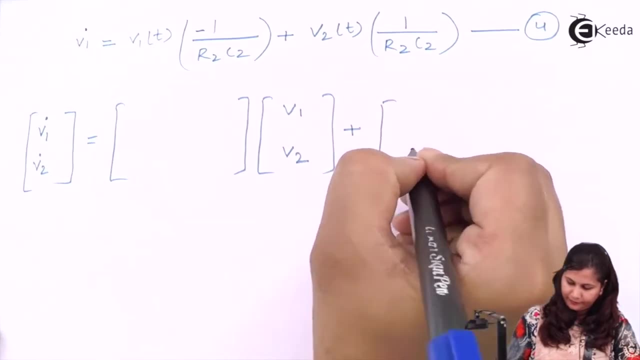 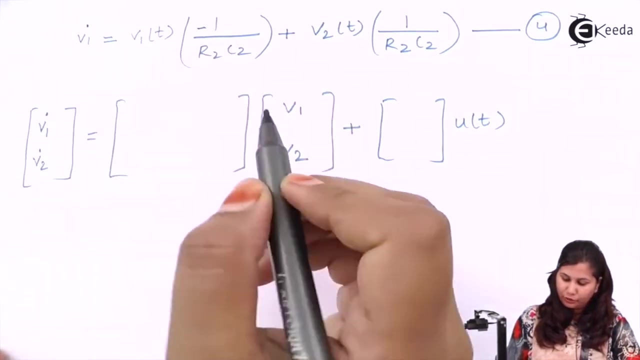 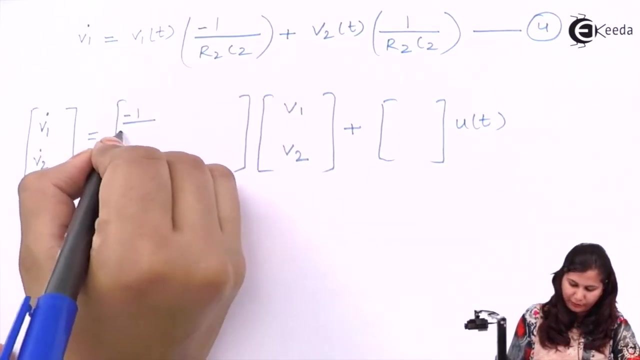 write here: minus V1 dot, It will be equals to our two state variables are v1 and v2 plus we have ut. So for v1 dot the equation is this: so the coefficient of v1 t will be minus 1 upon r2 c2.. So we will write here: minus 1 upon r2 c2.. The coefficient of v2. 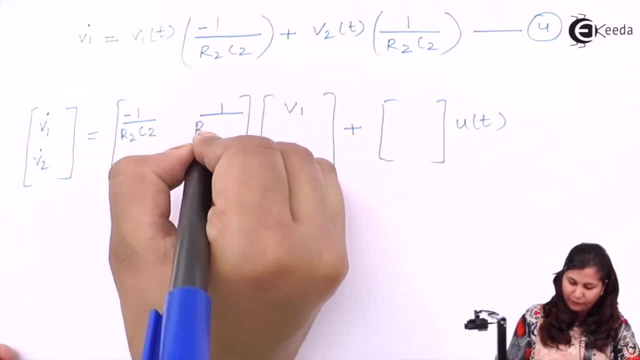 is 1 upon r2 c2.. Okay, Now we will learn more in a next video. Okay, Let's see, AD就是 1 upon r2 c2, so we can write 1 upon r2 c2 here. Then, from the third equation for v2 dot we have: 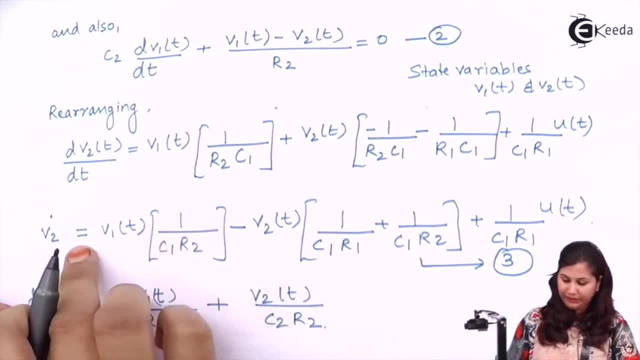 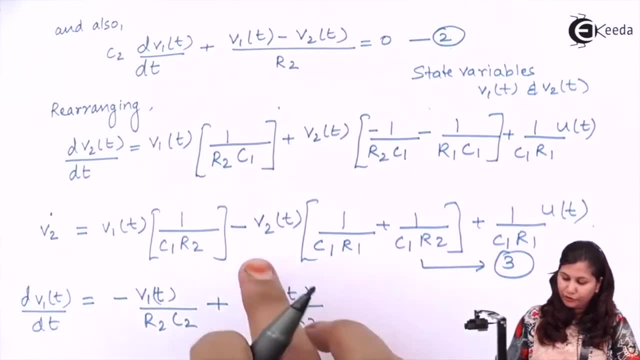 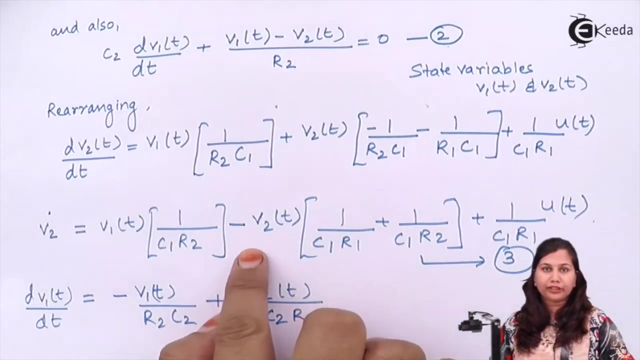 v1 t, as coefficient of v1 t is 1 upon c1 r2. so we will write 1 upon c1 r2.. Then the coefficient of v2 t is minus. this is minus sign. So the coefficient of v2 t, it is minus sign and 1 upon 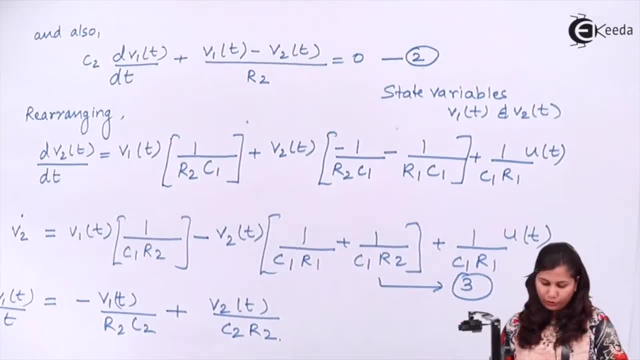 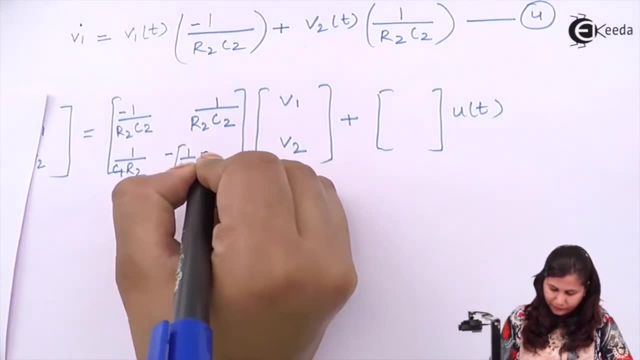 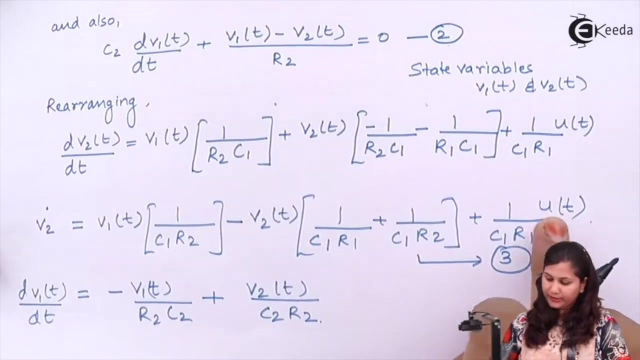 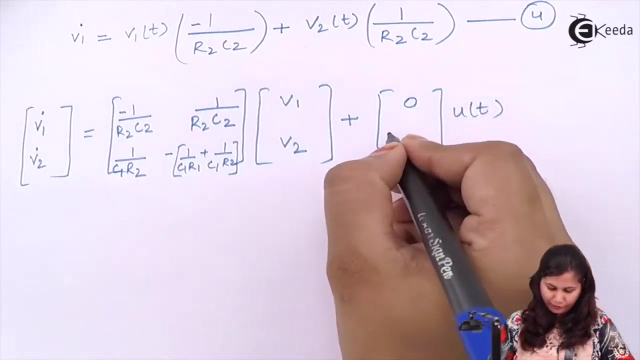 c1 r1 plus 1 upon c1 r2.. So we will write this here, minus 1 upon c1 r1 plus 1 upon c1 r2.. Then the coefficient of ut is 1 upon c1 r2.. In v1 dot ut was not present, so we will write 0 here, and here the coefficient is 1 upon c1 r1. 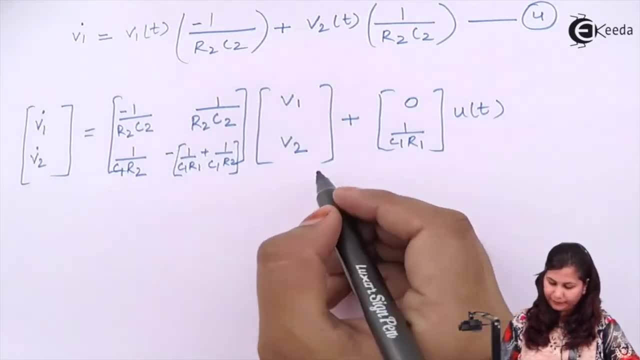 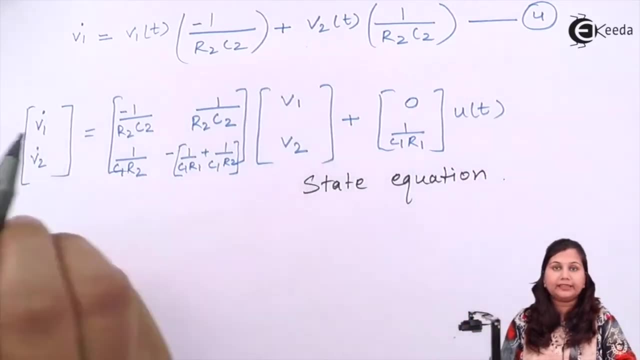 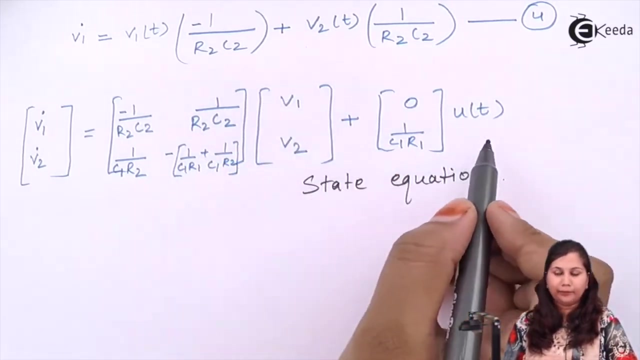 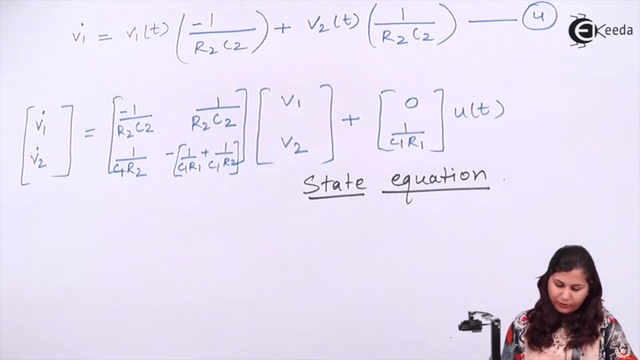 So this is our state equation. State equation because it is having the, it is defining the derivatives of the state variables as a linear combination of the state variables and the input. So it is defining the state variables, So it is called the state equation. Now we also know that the output- output is our v0 t. 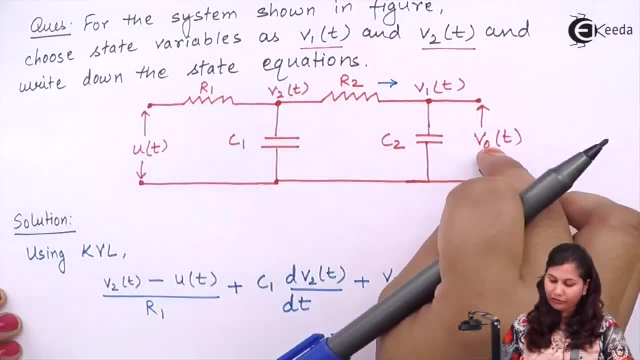 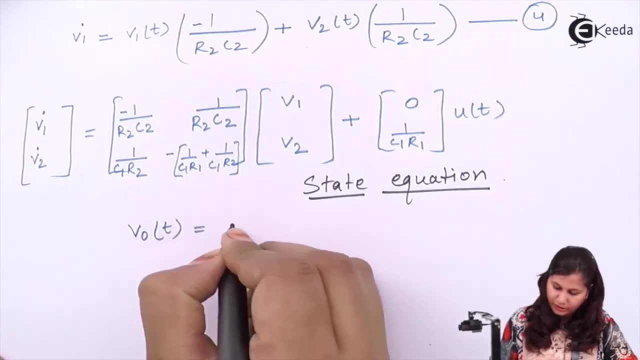 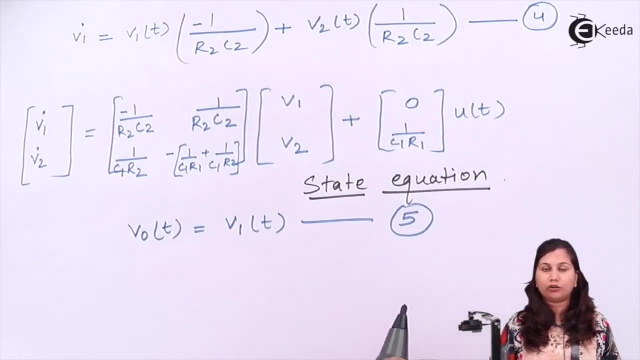 So in this diagram you can see that v0 t is equals to v1 t. So we have another equation: v0 t equals to v1 t. This is our fifth equation. So from this equation we can write the output equation. So output is what v0 t. 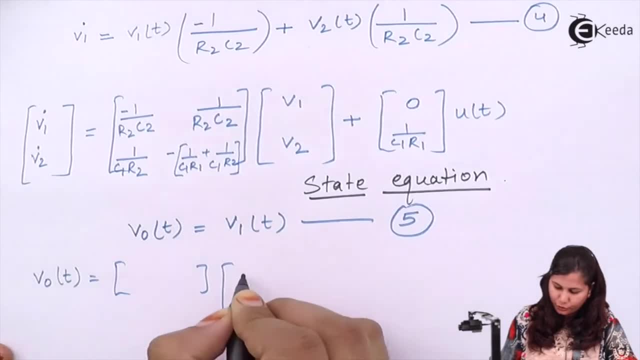 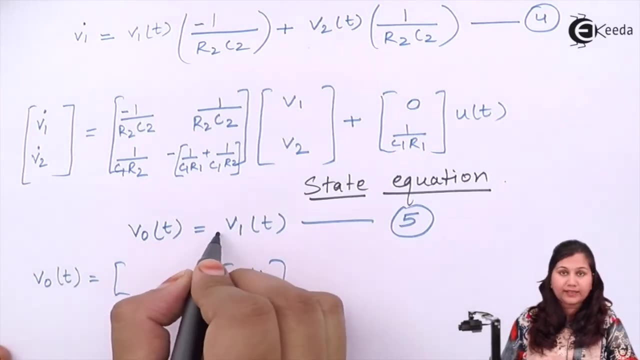 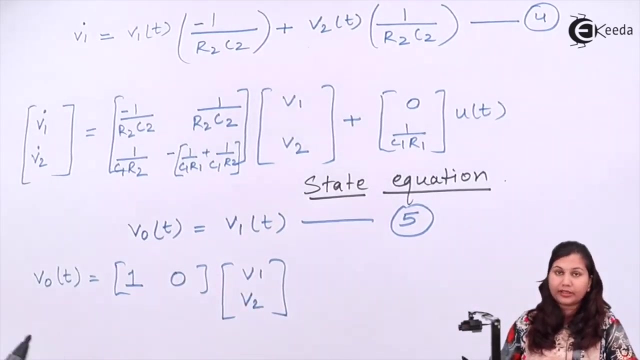 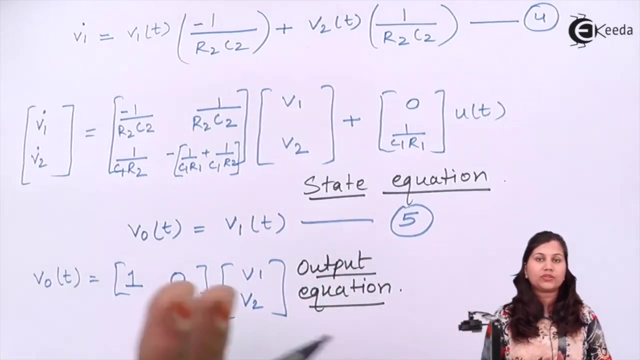 The two state variables are v1 and v2.. So v1 is coefficient, is 1. So we will write 1 here, and v2 is not present, So we will write 0 here. So this is our output equation. So these two equations, state equation and the output equation, they constitute the state model. 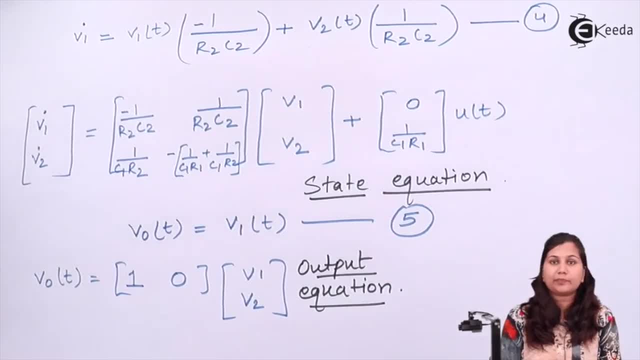 of the system, or we can say that it is the state space representation of the system. So in this way we can find out the state space representation for any type of system We will choose. we will write the equations for the state variable. So we will write the equations for the state variable. 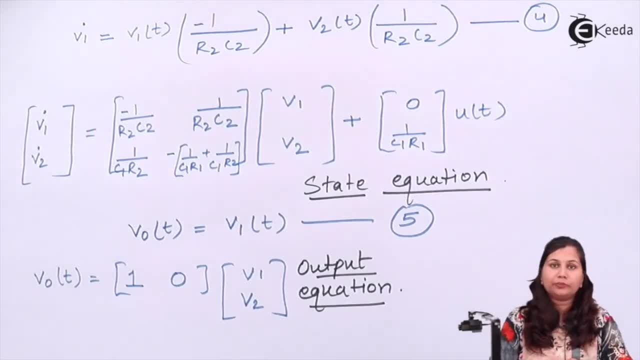 Derivatives of the state variable and the output variable. So I hope this problem is clear to you. Thank you.